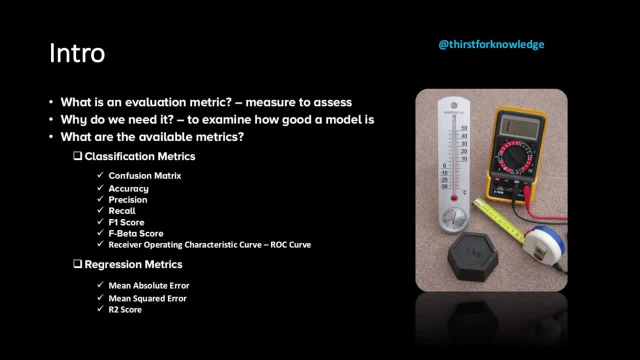 Yeah, it's pretty straightforward. We measure it in liters, right? And you can also see a couple of measuring instruments here- the right side of the slide, okay so- which we use in our day-to-day life for different purposes. So, in a similar fashion, if we want to measure the performance of a machine, 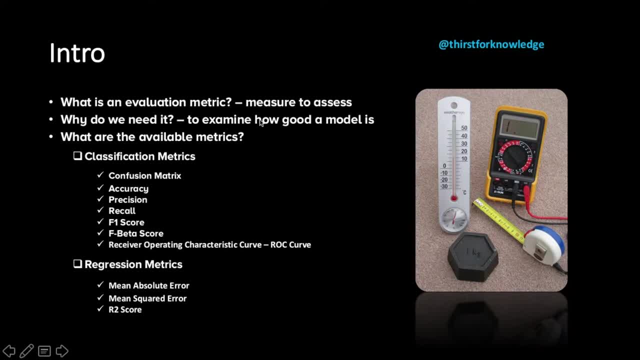 learning model or an algorithm? how do we do that? Okay, Are there any metric to help us with? Yes, We have quite a few metrics, As we all know that we mainly deal with two types of problems in machine learning. They are nothing but. 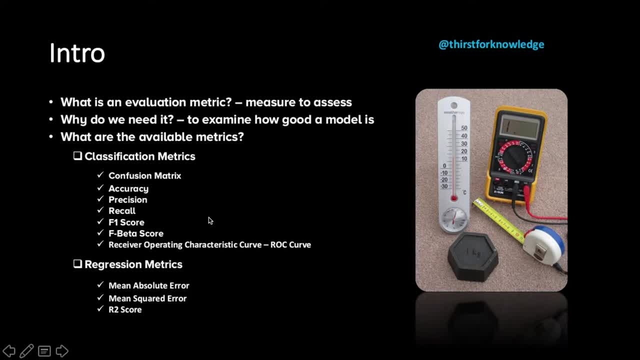 the classification and the regression problems. The classification problems are perhaps the most common type of machine learning problems. The classification problems are يعرضy 놓ing common type of machine learning problems and, as such, there are a myriad of metrics that can be used to evaluate predictions of these models. 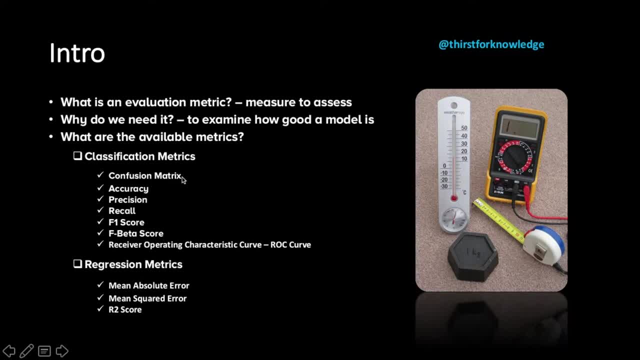 You can see a couple of metrics listed out here for the classification problems like confusion, matrix, accuracy, precision, recall, F1 score, Fbeta score and receiver operating characteristic curve, which is nothing but the OVC curve. So along with these metrics we do have a bunch of metrics to assess the performance of a 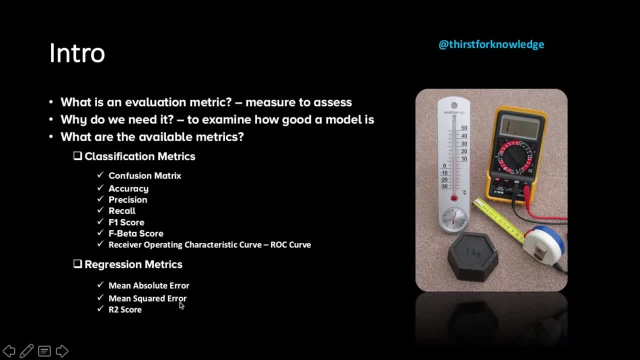 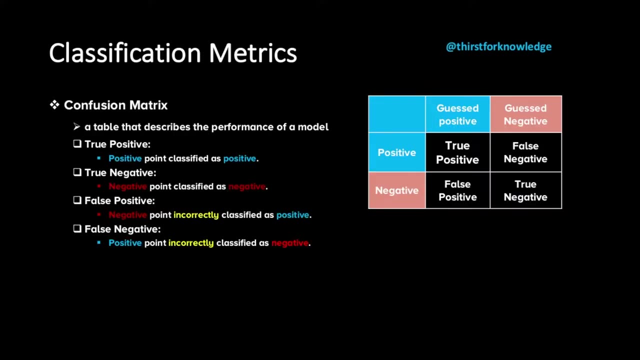 regression model, Such as mean absolute error, Mean squared error And R2 score. Alright, We are gonna discuss more about these techniques soon, So let's jump into the classification metrics. First, we are gonna discuss about the confusion matrix. Yeah well, so what is a confusion matrix? 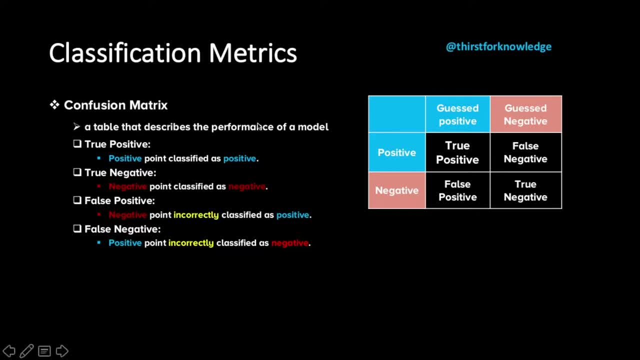 Confusion matrix is nothing but a table which describes the performance of a learning algorithm or environment. It is a model. Before we deep dive into the confusion matrix, let me introduce you to a few key terms which we are gonna use to construct the confusion matrix. 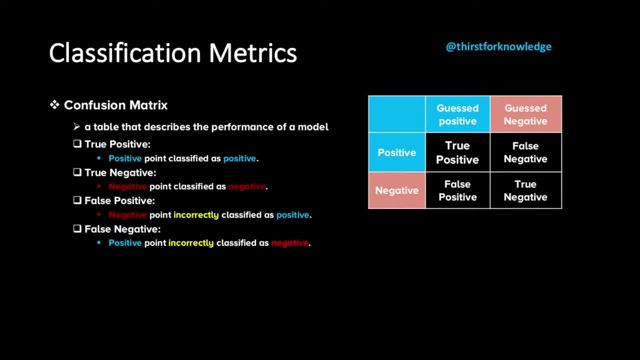 Okay, So let's go one by one. The first one is the true positives. True positives are nothing but the points that are positive and model correctly classified as a positive. That is nothing but a true point being classified as a positive point by the model. 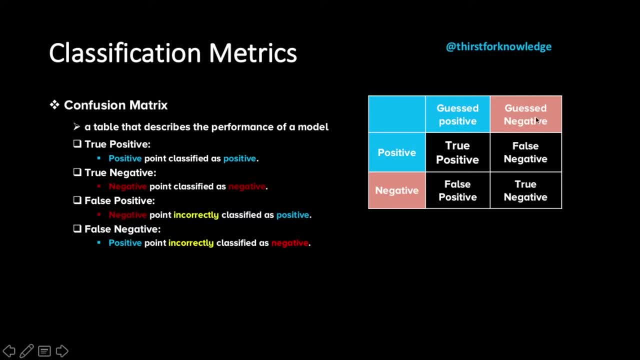 Similarly, true negatives are the points that are negative and model correctly classify them as a negative. In short, if I have a true, positive point- Sorry, If I have a positive point, If my model classifies it as a positive, So positive is my input and it is classified as a positive again. 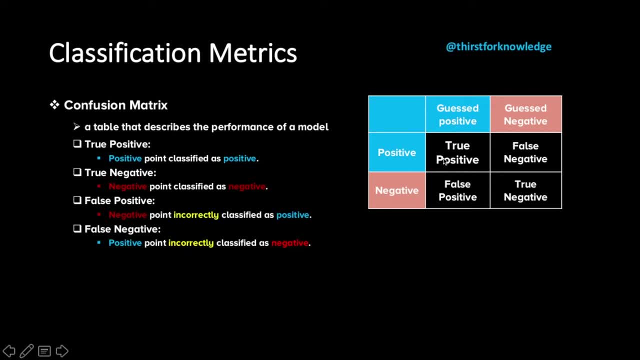 So that is my output. That is nothing but the true positive. Similarly true negative is nothing but like a negative point being classified as a negative point by the model. Similarly true negatives are the points that are positive and model correctly classified as a negative point. 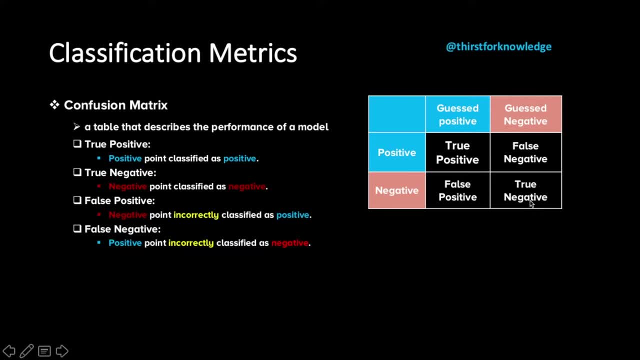 Say: if I have a true positive point, okay, so it is clear. I think there is no logical. it's not that much difficult to understand, right? so true, positive and true negative are straightforward. I have a negative point. if my classifier classifies it as a negative, true. 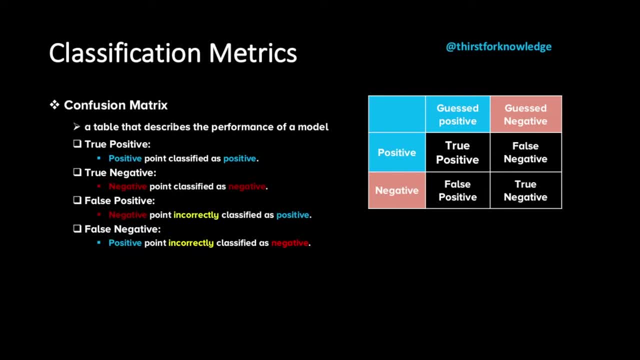 negative. if I have a positive point, if my classifier classifies it as a positive, then I call it as a true positive. very clear, right? okay, now check the false positive. yeah, false positives are nothing but the points that are negative. okay, but the model incorrectly classify them as a positive. okay, listen. 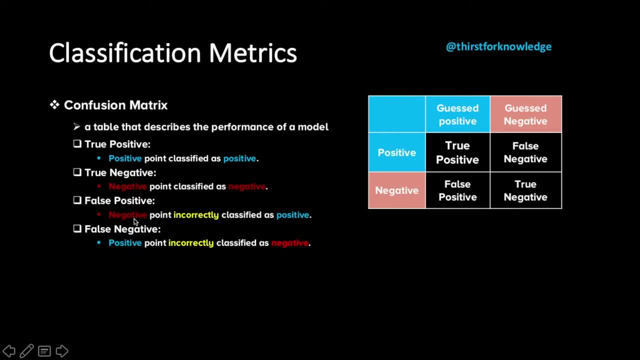 to this carefully. this is a tricky one. false positive is nothing but the point at the point. I have a negative point, but my model classified it incorrectly as a positive. okay, so we call this type of points of the, this type of scenario as a false positive scenario and similarly. 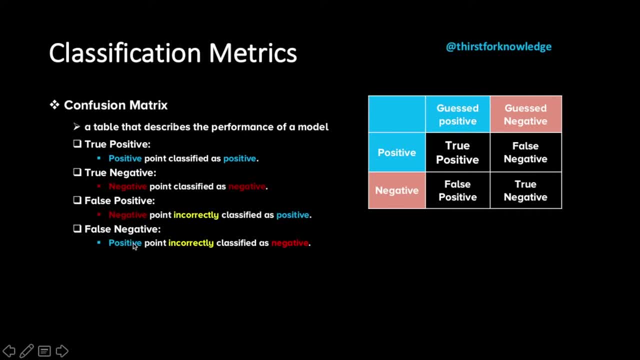 false and negative points that are positive, okay, but model incorrect classify them as a negative, which is nothing. but I gave a negative point as input but my model classified it as a positive- okay. but don't worry if you don't, if you didn't understand or if you didn't get these terms, because 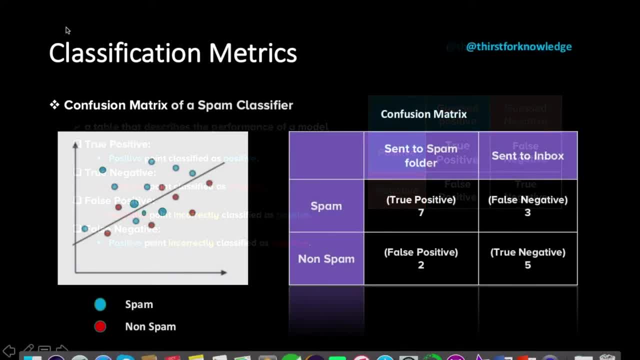 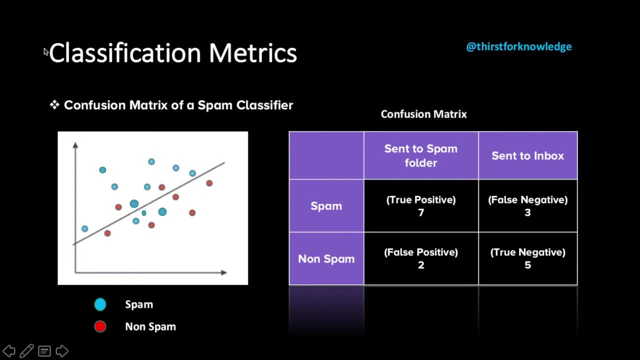 I'm going to explain these terms with an example. so now let's look at and analyze the confusion matrix of the spam classifier. so first examine the model when a blue point represents a spam mail and a red point represents a non spam mail, and also remember that classifier sends a 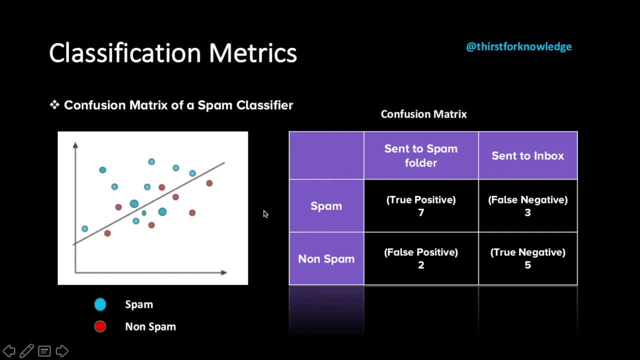 mail to spam folder if it's classified as spam and it sends all of the non spam mails to the inbox. okay, all right, let's find out the true positive count of this classifier. so, as per the definition which we have seen earlier, true positives are nothing but the points that are positive, and 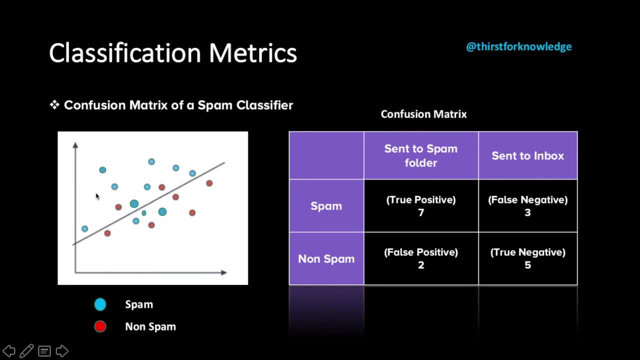 model correctly classify them as positive. that is nothing but the number of mails classifier has sent to spam folder that were originally spam see. similarly true negative count is the number of non spam mails that classifier sent to inbox that were originally not spam. so the true positive count of this 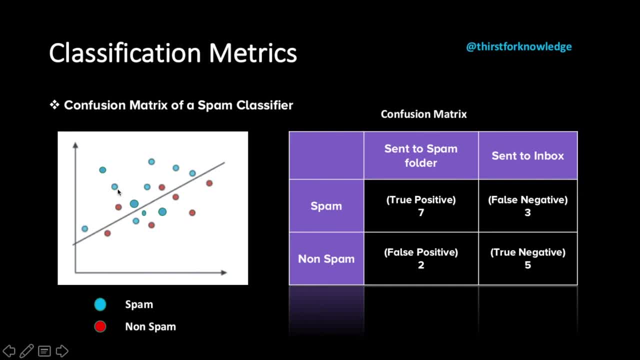 classifier is one, two, three, four, five, six, seven. okay, so the total counter the true positive counter, the classifier is seven and the two negative count is five. okay, when it comes to the false negative, which is nothing but the negative count, and the true negative count is 5. okay, when it comes to the false negative, which is nothing. 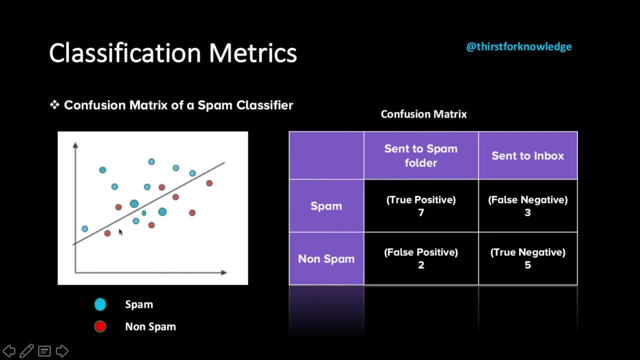 the number of spam mails sent to inbox, that is, a number of mails that are misclassified as non-spam but were originally spam. so the false negative count is three, and similarly the false positive count is the number of non-spam mails classified as spam and, as a result, sent to the spam folder.